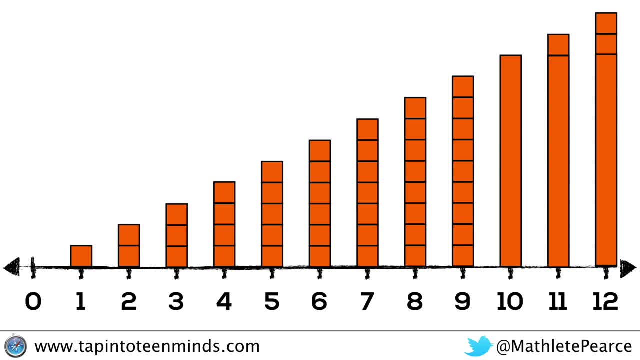 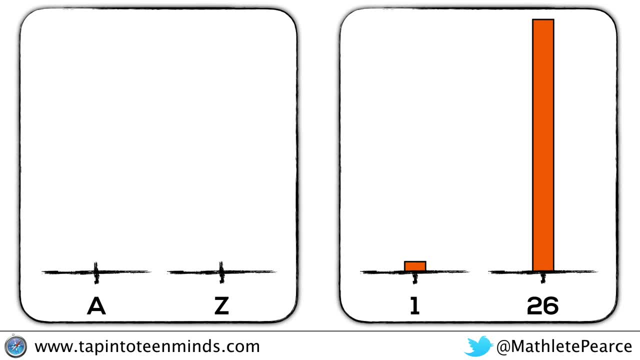 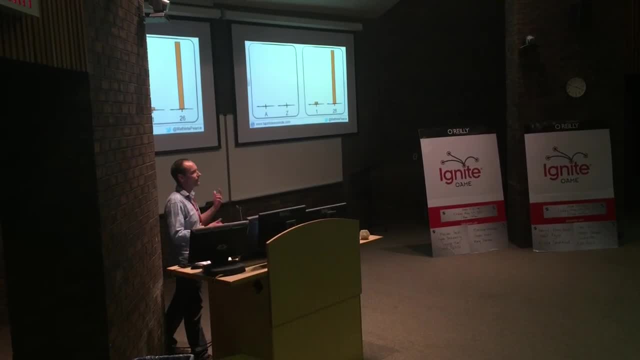 magnitude. the numbers 1 and 26 have a very different magnitude And over time students must build this understanding to know that actually 26 is 25 units bigger or 26 times as great as, or that there's all kinds of other relationships that are existing within this idea. 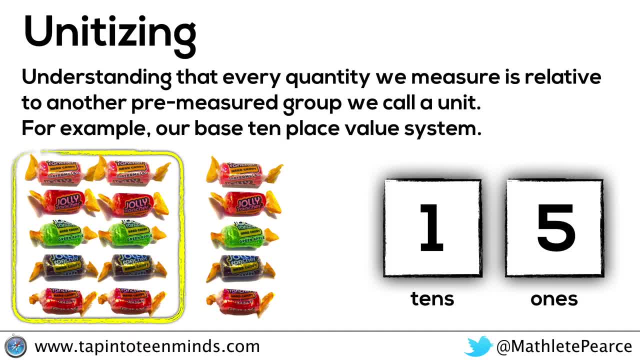 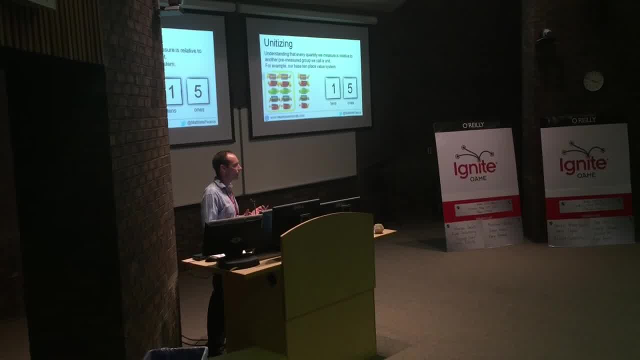 Now, don't even get me started on unitizing. With unitizing, students have to start counting groups of objects. And now this is really important- When we think about place value and when we start making the leaps towards multiplication and division, and when we start talking about multiplication and division, 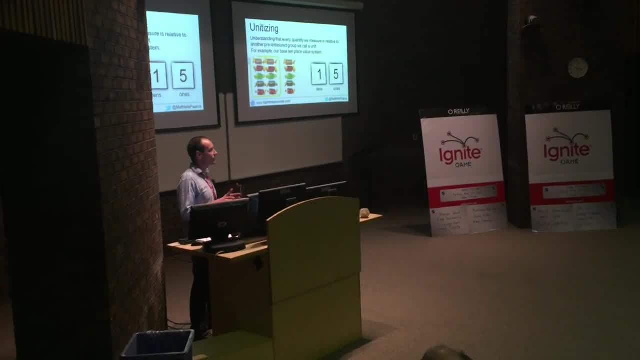 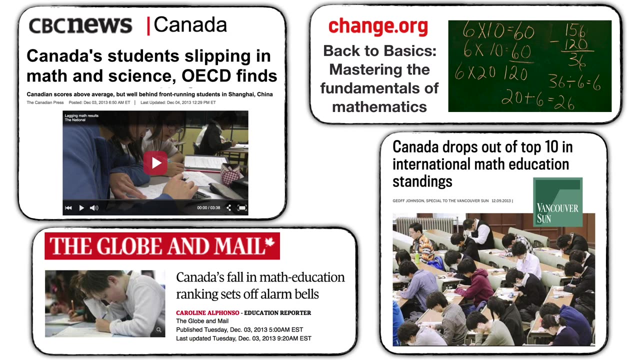 you'll probably think about math facts And when you think of the groups in the media that are constantly distracting our elementary teachers about math facts and back to basics, they can be negatively influenced to start doing things that people tell them they should be doing instead of what they know is right. 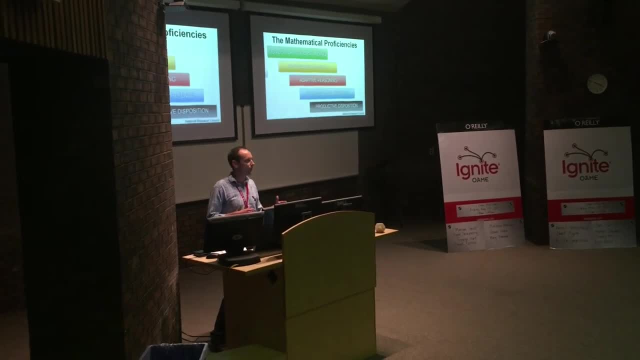 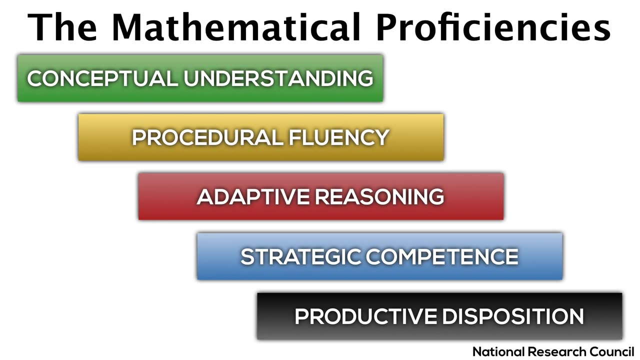 If I believe that math proficiency is memorizing math facts, rules and procedures, then I might also believe- and without doing that, without conceptual understanding to underpin these ideas, then I might also believe- that counting is as simple as just resetting your alphabet. 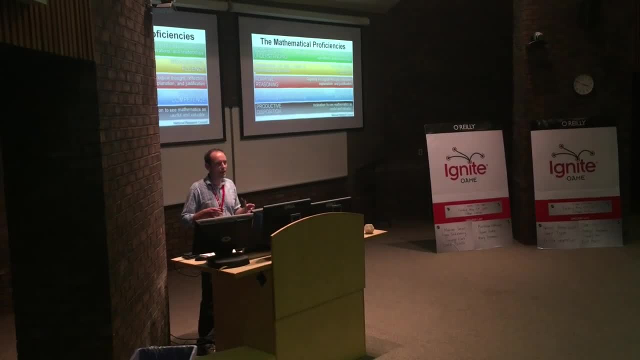 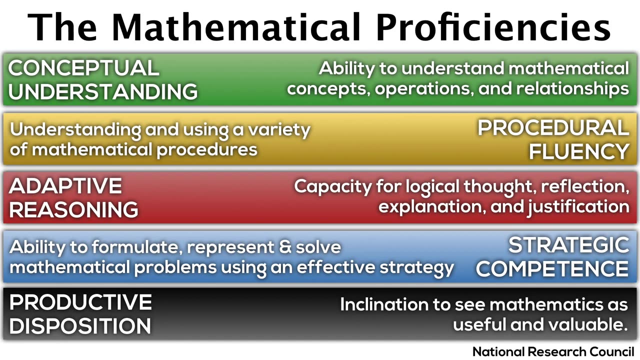 Right Now. don't get me wrong. I think anyone interested in math education wants students to have automaticity of math facts, but I think the real debate is how we get students to that automaticity Alright. So when we're doing this and we're building this automaticity, we need to be thinking about 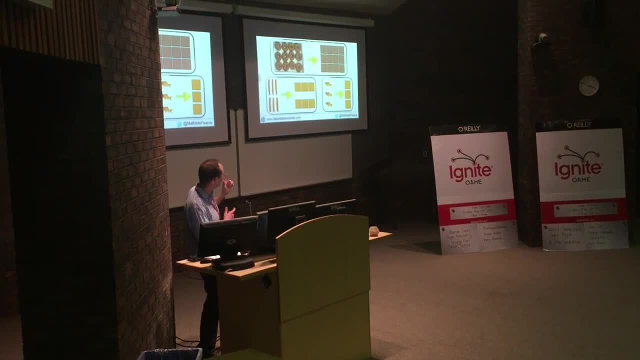 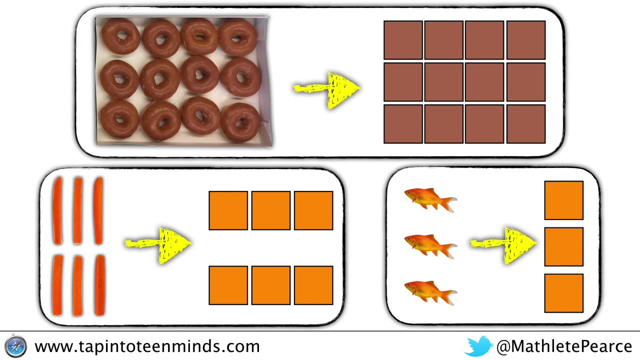 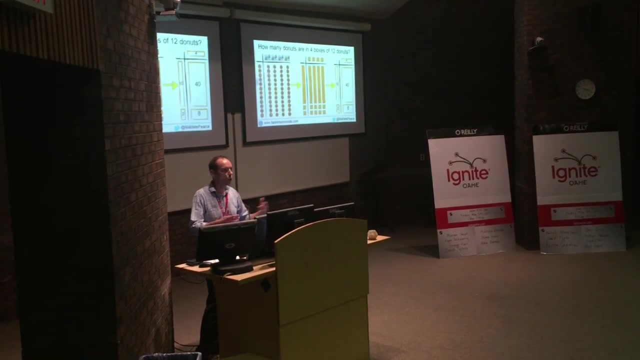 how and what and why we're doing what we're doing Now. our elementary teachers are great at doing this stuff. They know that students thrive on context and they thirst to hold real objects in their hands, And over time, students will start using square tiles and other manipulatives to represent donuts or carrots or goldfish. 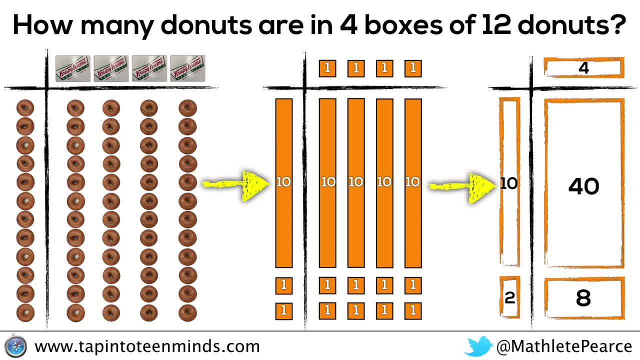 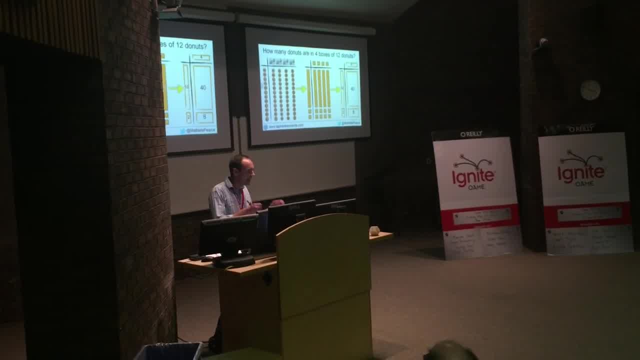 And in time students will become so comfortable with those representations that they might start drawing and start pushing those manipulatives away because they're too cumbersome or time-consuming. And then, and only then, is when the teacher should start really pushing that symbolic and that structure. 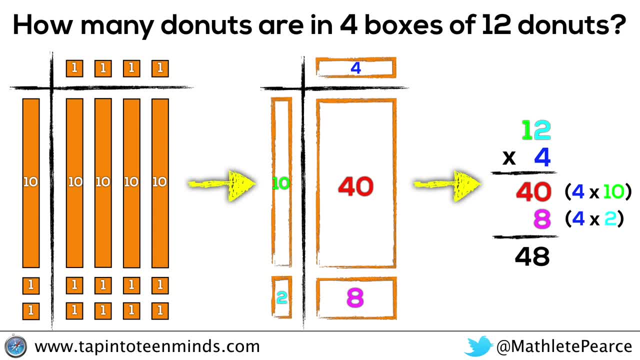 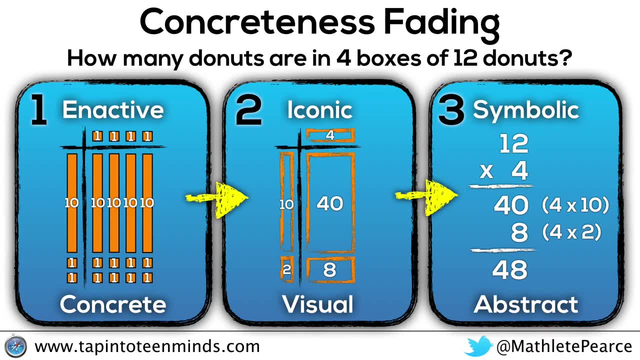 of the mathematics starting, leading them towards procedural fluency and towards that automaticity. Now, what I'm talking about is something called concreteness fading, And as a secondary teacher, this is a brand new idea that could really help me when I had students that were struggling in my courses.